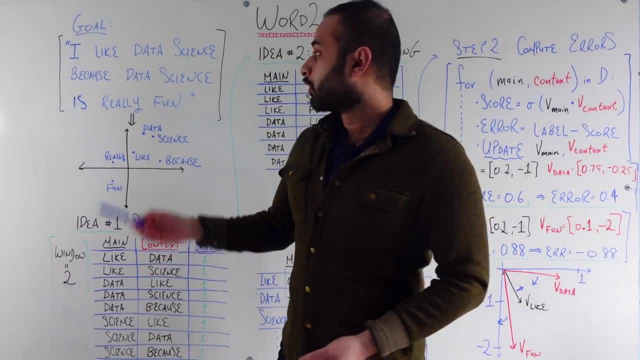 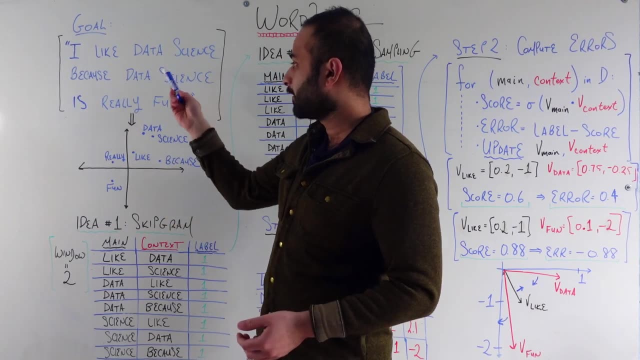 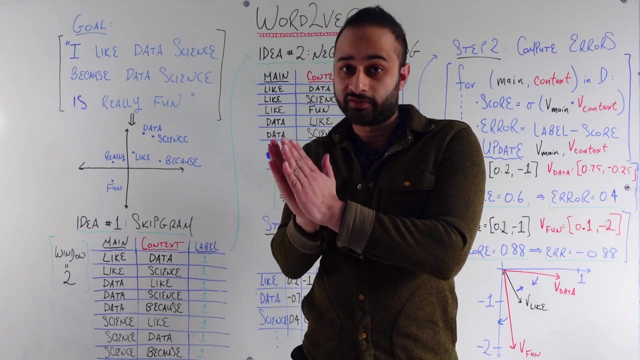 one vector for each word, such that words that often appear close to each other many, many times, like, for example, data and science, are close to each other, and there's multiple instances of that. that should translate, at the end of the day, into getting the vectors for data and science to be literally close to each other in the vector space. 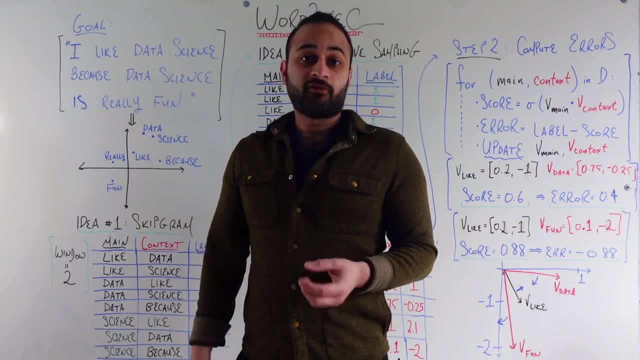 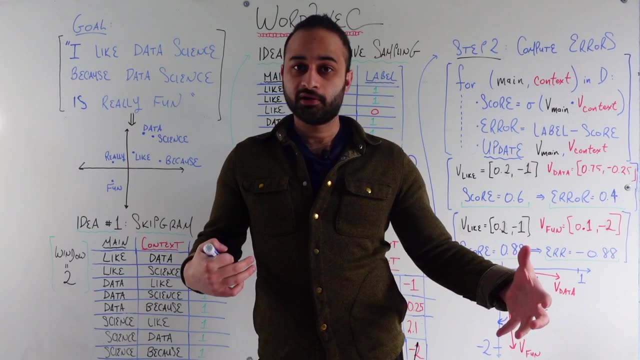 And so we'll see how Word2Vec achieves this very cool goal. But before we do that, we need to get a couple of ideas across, because currently we're just looking at a string of words. We need to turn this into some kind of structured data so that Word2Vec can do its thing. 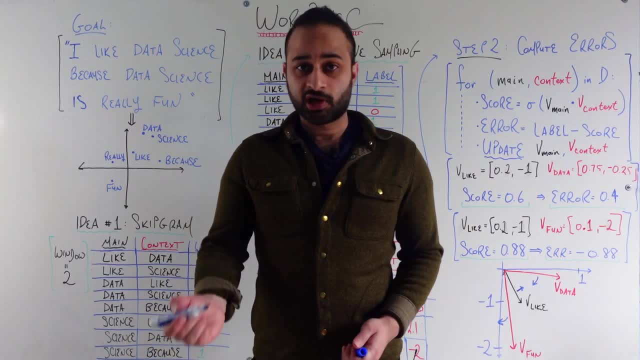 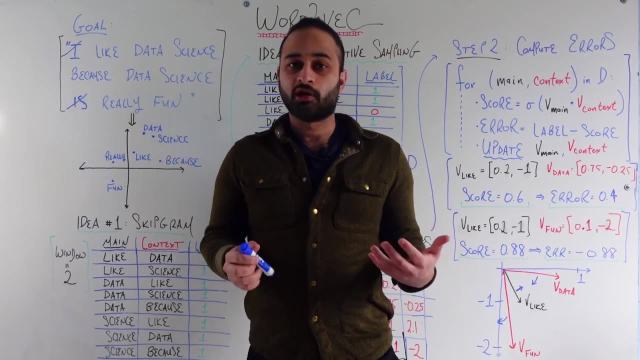 The first thing we actually need to do is delete some words called stop words. So, for example, I and is are kind of just these common, everyday, no real meaning words called stop words And you could leave them in there. it's probably not going to interfere too much. 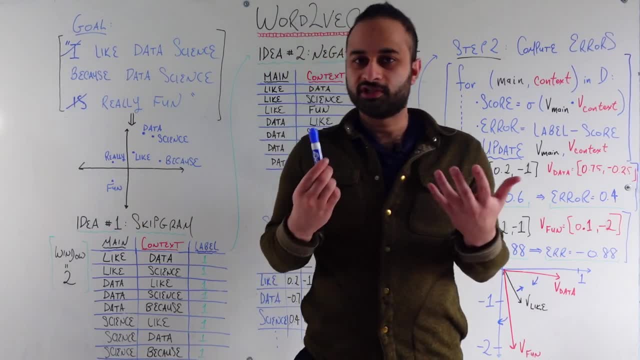 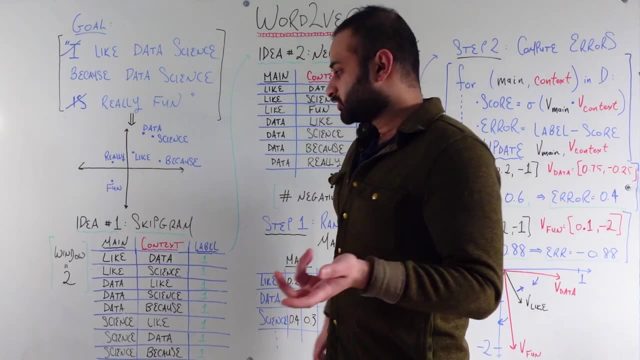 but typically we remove them because we're not interested in those common words. we're more interested in the true words in our sentence. so that's the first step. Then big idea number one is called skip gram. This is pretty simple. we first pick a window size. for example, let's pick window size 2,. 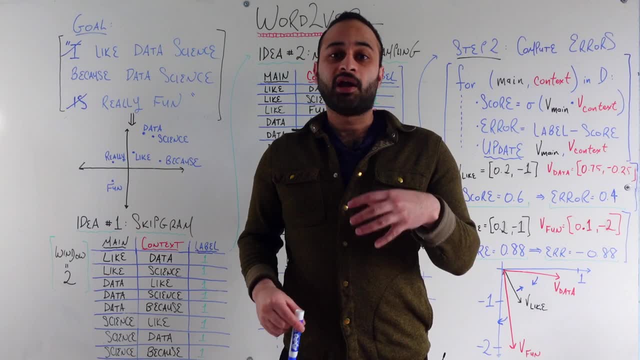 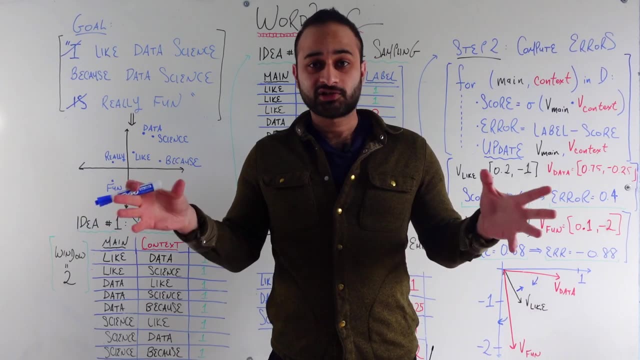 and then we visit each and every word that's in the sentence and we ask who are the two words that are to your left and who are the two words that are to your right. We're going to call that your context or your neighborhood, and we're going to record all of that into this table here. 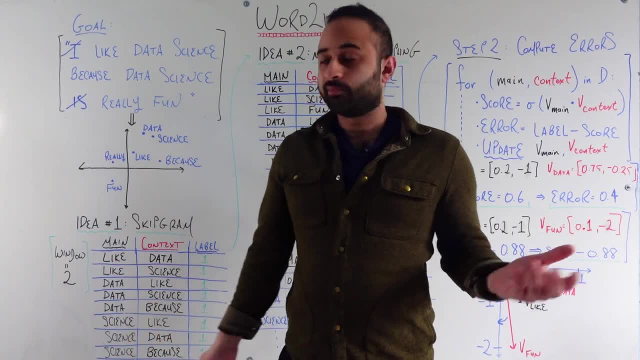 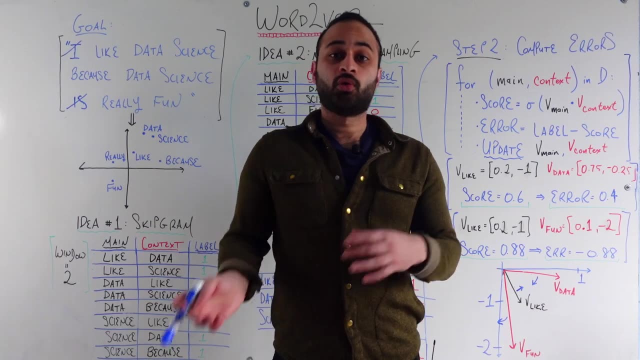 And that idea is called skip gram. So let's just go through a couple of examples. The first thing we'll look at is the word like, and we'll talk about who are the two words to your left. well, nobody on your left, but who are the two words on your right? 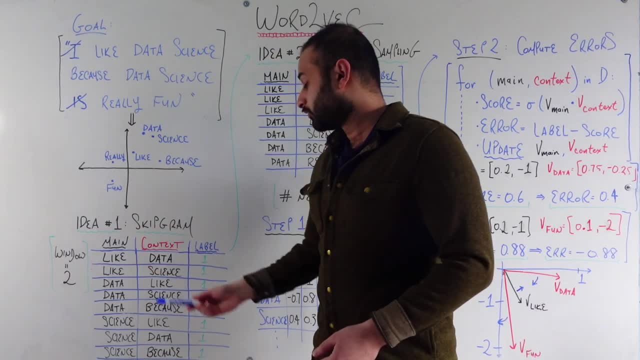 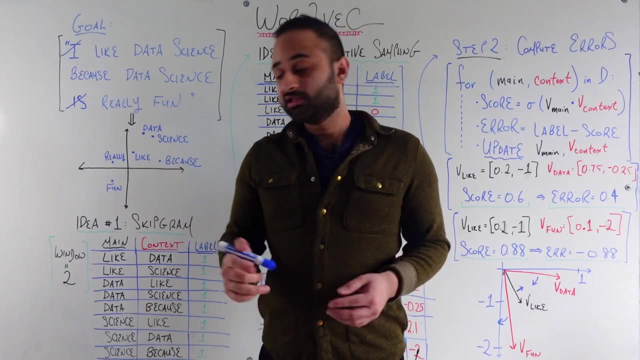 Well, that's the word data and the word science, and that's why the first two things we record are like and data and like and science, and they both get a label of 1, which means that these, this main word and this context word- 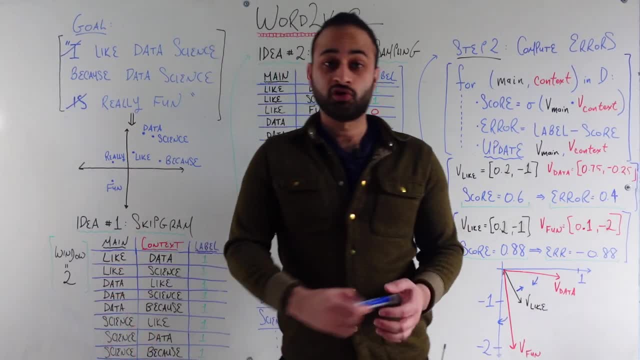 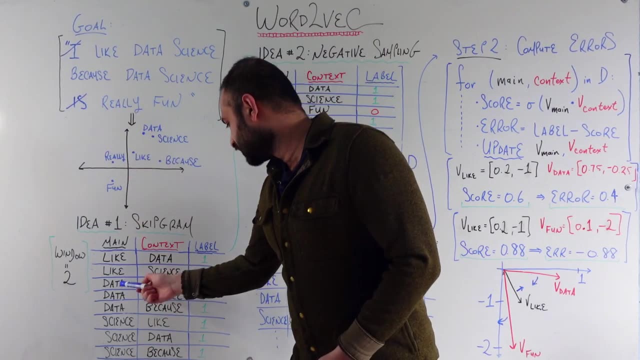 do appear next to each other within a window size of 2.. And we can just keep going. So we get the word data. who are the two words to your left? Well, just the word like here. so we get data and like. 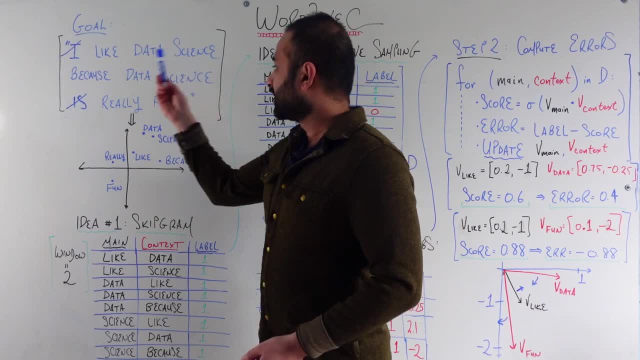 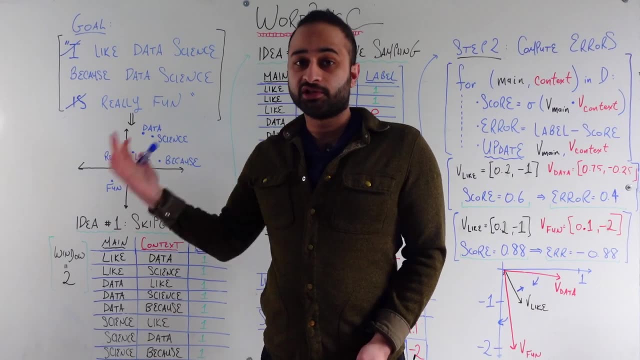 Who are the two words to your right? Well, it's going to be science, and because, science and because- and those get labels of 1 as well, And we just keep going. we construct this for the entire sentence or paragraph. Now, why can we not stop here? 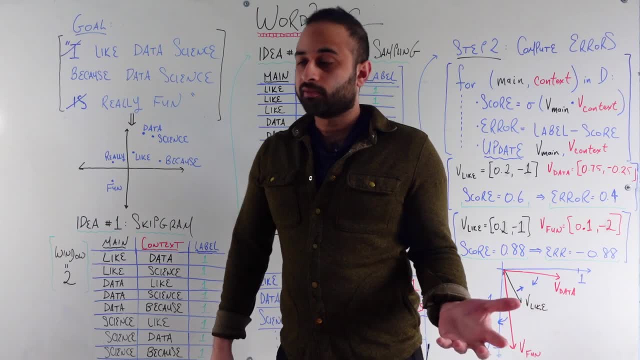 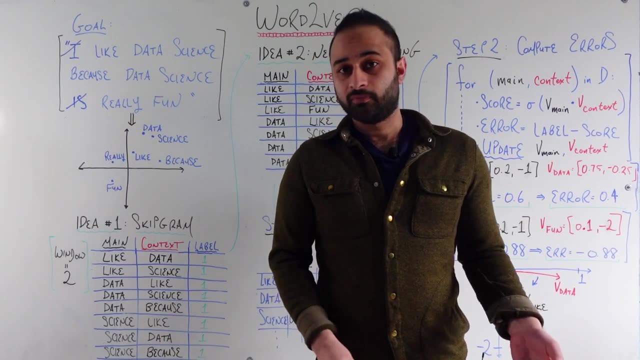 Why isn't this enough to just feed into whatever method we're going to use? Well, you probably noticed, but all the labels are 1. And we can't really do much good machine learning if all of our labels are the same. That's like trying to build an image classification method. 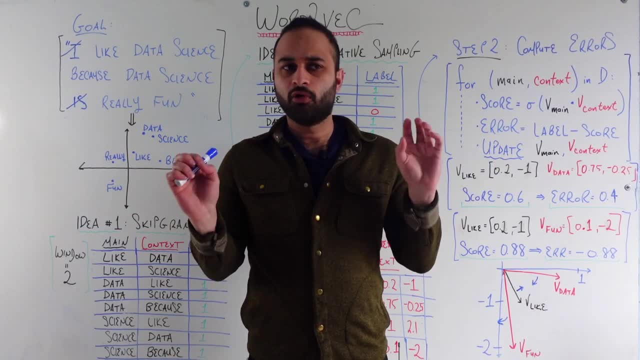 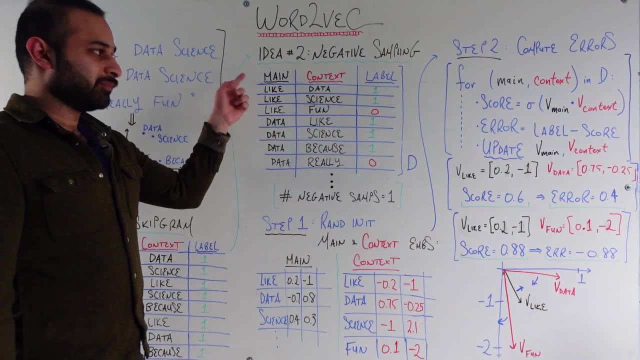 that's supposed to tell cats apart from dogs, but you only feed it pictures of cats. Probably not going to do a very good job. So that brings us to our next big idea, which is called negative sampling. Negative sampling is pretty simple. 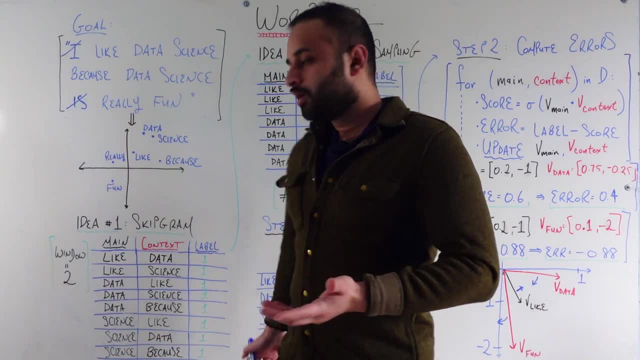 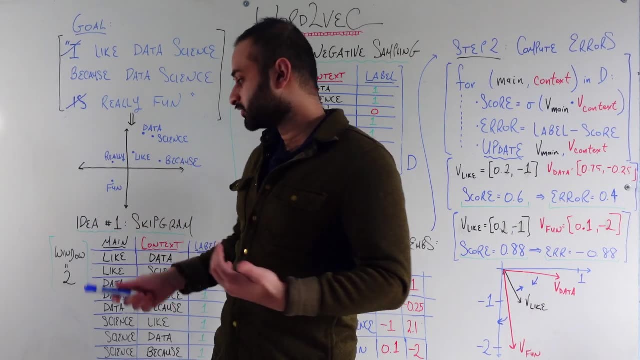 We're just trying to fix this issue that all of our labels are currently 1, by introducing some examples of main and context words which actually are not next to each other, not within a window size of 2. And so we just pick a number of negative samples per main word. 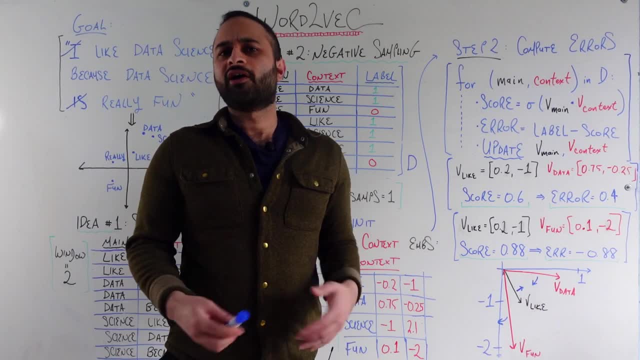 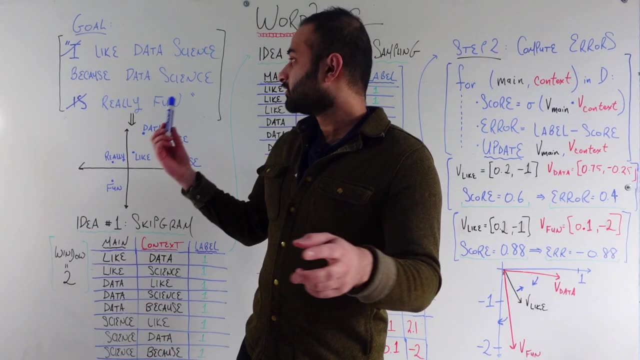 here we just picked 1 to keep things simple, but typically you'll have more than this, so it has many different examples to learn from, And so, for example, the word like and the word fun, if you look within these sentences, don't appear within 2 words of each other. 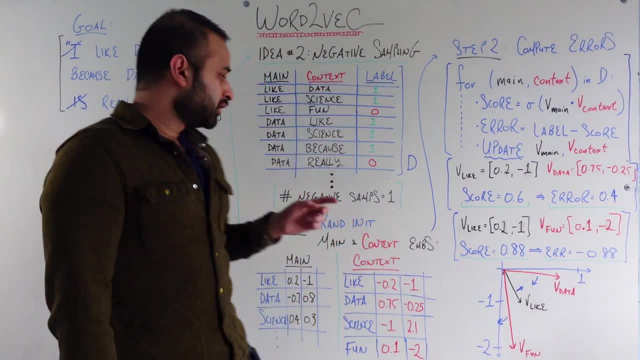 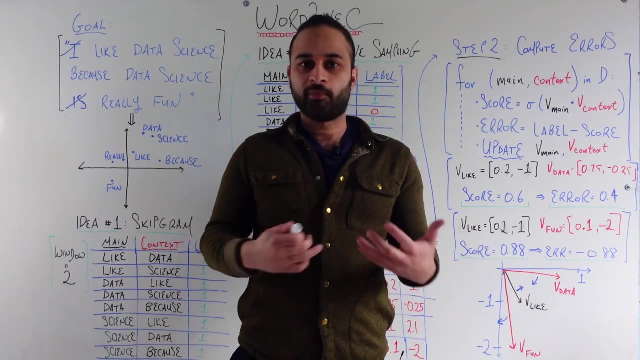 and so we introduce that as a negative sample with label 0. The word data and the word really. here we're talking about the first word, data, because you have duplicate words- data- so you kind of talk about them individually. But the first word, data, does not have the word really within 2 words of its left. 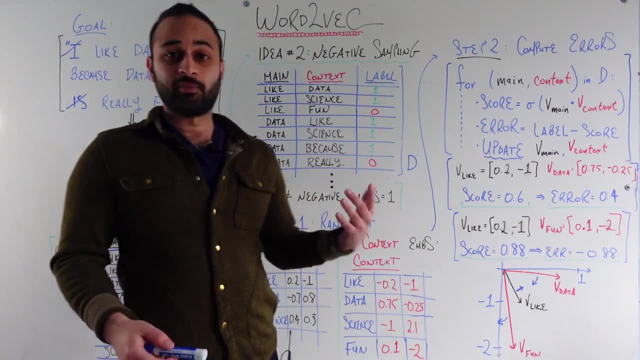 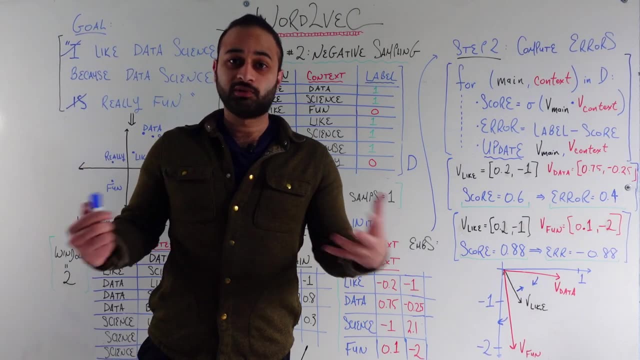 or 2 words of its right, and therefore we also give this a label of 0.. Now we're ready to go. Now we have positive, we have negative labels, and this whole data tells the story about which words are close to each other. 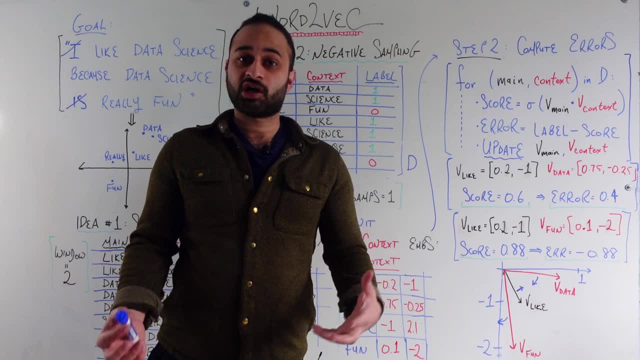 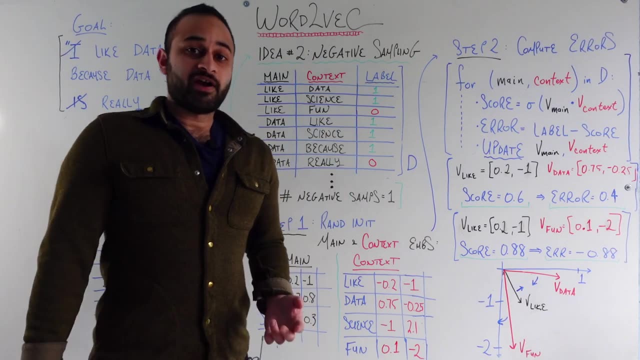 so Word2Vec should be able to figure out these patterns, and let's talk about how Word2Vec actually works now. So the first big idea we need to get across- and for me, the most confusing part of Word2Vec- is the fact that we actually have 2 sets of embeddings. 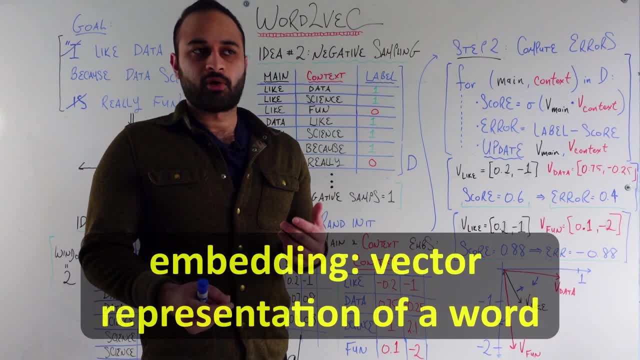 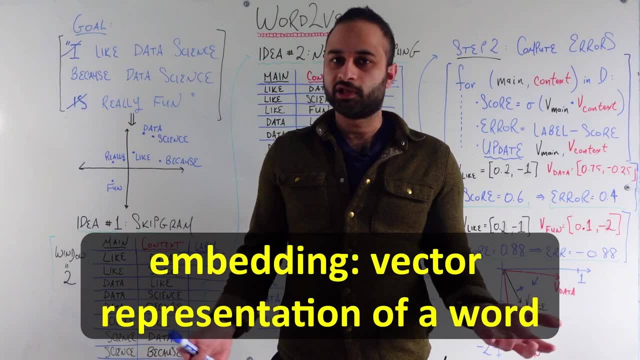 And, by the way, a embedding. you'll see this word thrown around everywhere in natural language processing. But an embedding is just a vector representation of a word. So we can use this word vector or the word embedding kind of interchangeably. 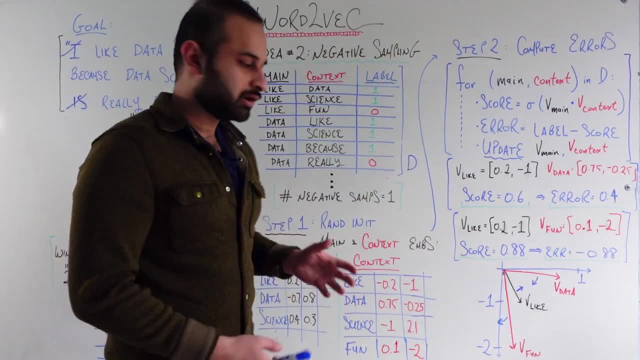 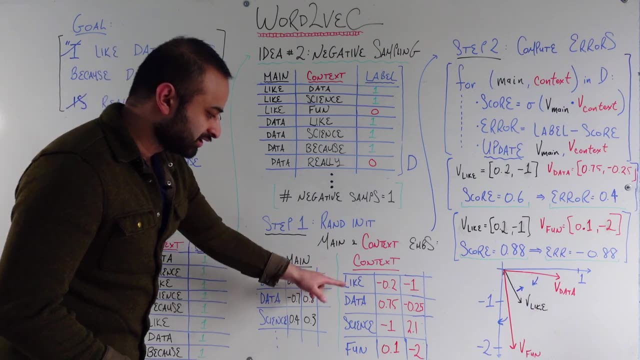 it's just that embedding is more context specific to natural language processing. So the confusing part of Word2Vec for me when I first learned it is that for each word, for example, the word like data science, like data science- we don't just have 1 vector that we're going to be updating and hopefully getting to be better. 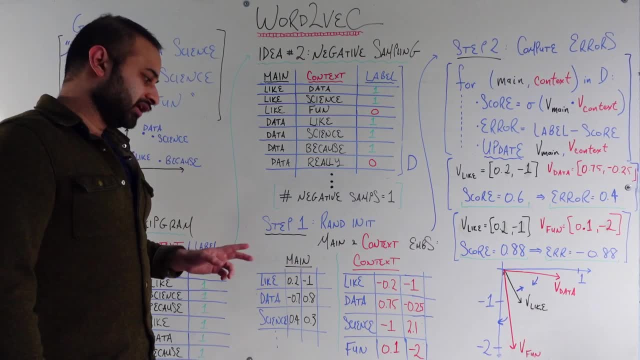 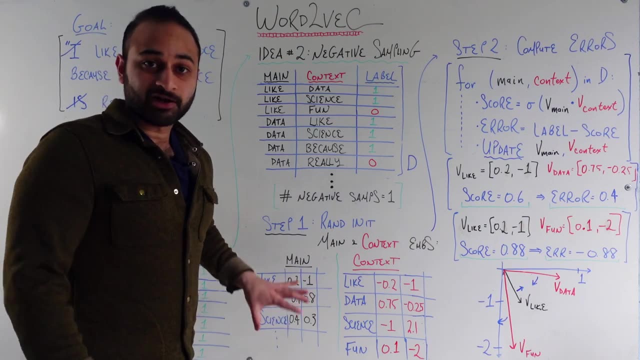 we have 2 vectors for each word that we're going to be updating. The first vector for each word is going to be is called the main embedding, and those are the embeddings at the end of the day that we're actually going to keep. 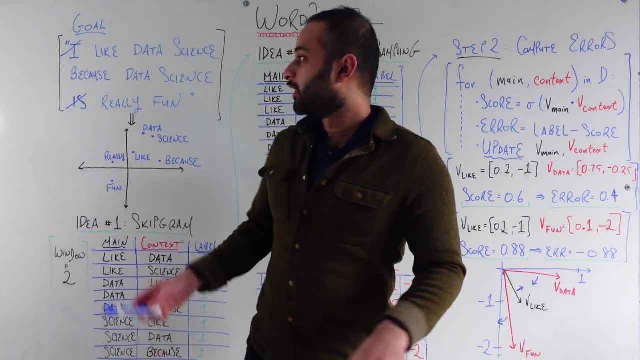 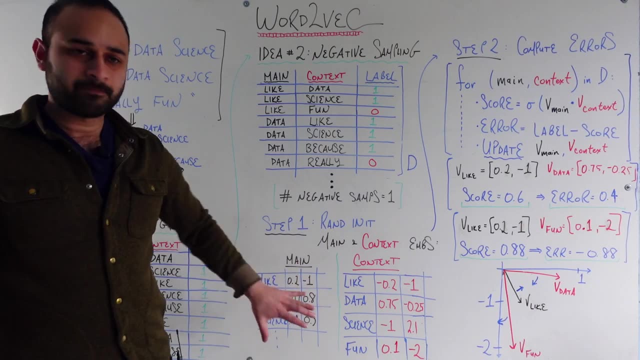 and those are going to be the answers to our initial question about how do we take each of these words and project it into some kind of vector space. So that's pretty clear. that's the answer to our eventual question. So what the heck are these other embeddings? 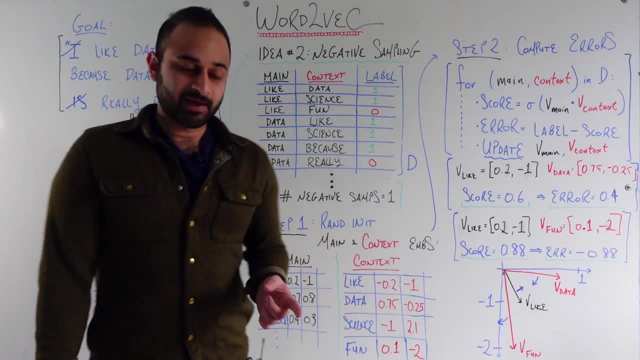 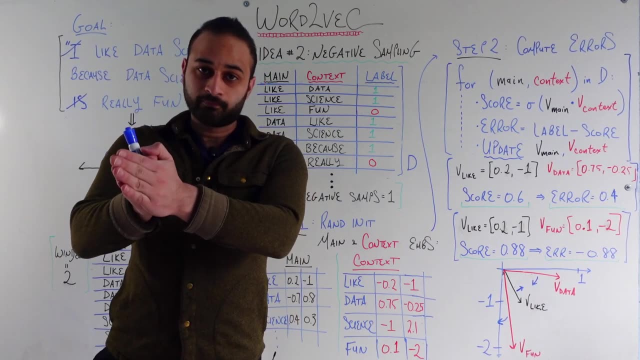 These are called context embeddings, and the way to think about those is that the main embeddings tell us about what's the vector representation of a word. if that's the current word we're looking at, The context embedding of a word tells us what's the vector representation of a word. 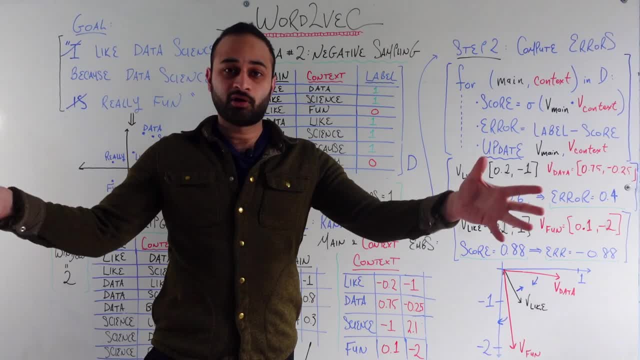 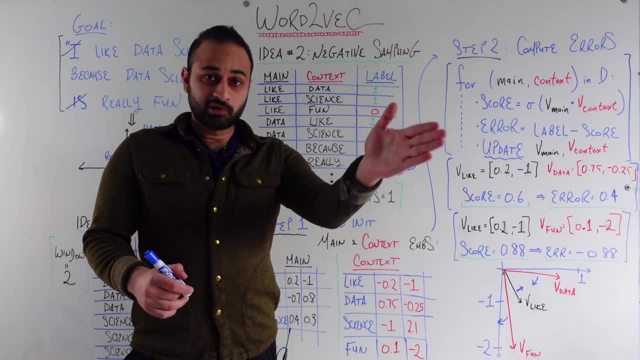 if it is the context, if it is the kind of neighborhood of a different current word we're looking at. So hopefully that kind of makes sense. but the main embeddings tell us about that's the word we're looking at and this is the vector representation. 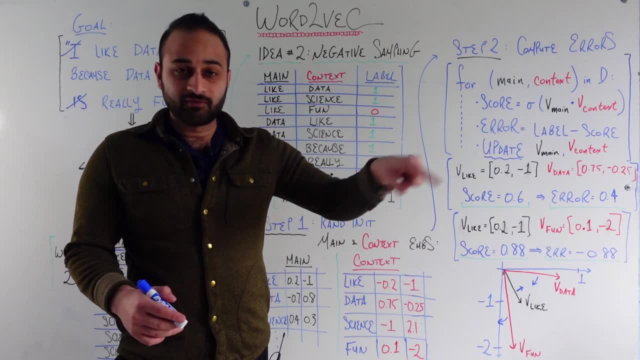 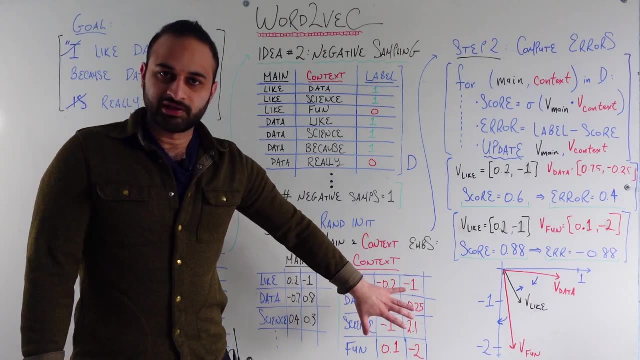 The context embedding tells us about. if this is kind of a neighborhood word, then how do we represent it as a vector? And although we're just going to keep this at the end of the day and we'll just discard these, we don't really need them. 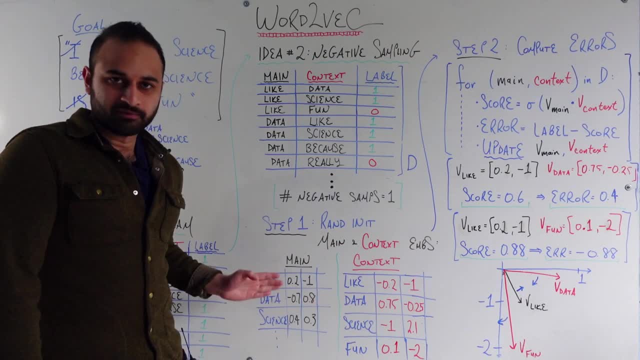 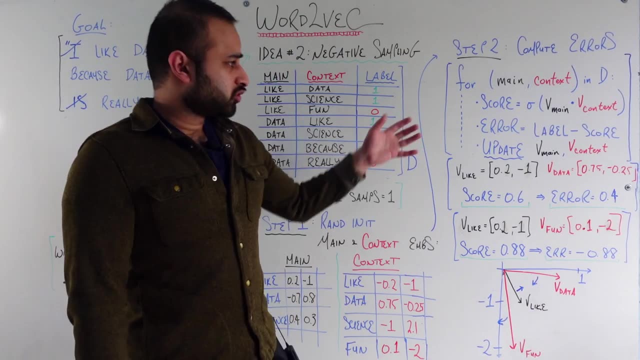 we need to carry these around in order to successfully update them. So that'll make much more sense now when we talk about the actual algorithm of Word2Vec. So you can see it's pretty short. it's not going to take much for us to explain it. 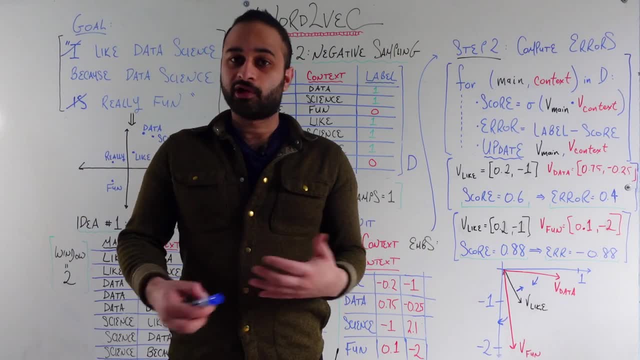 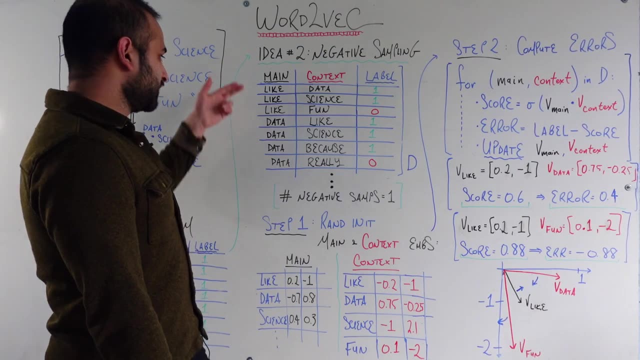 and we actually have a real example with real data that we'll talk about in parallel, so we can actually see this in practice. So the outer for loop says: for every row in our data, D. so we're basically just going to walk down this entire data set. 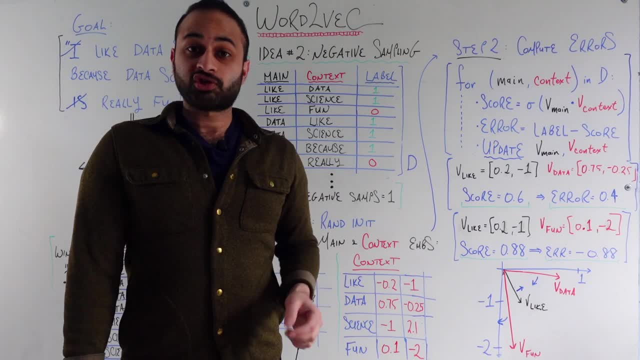 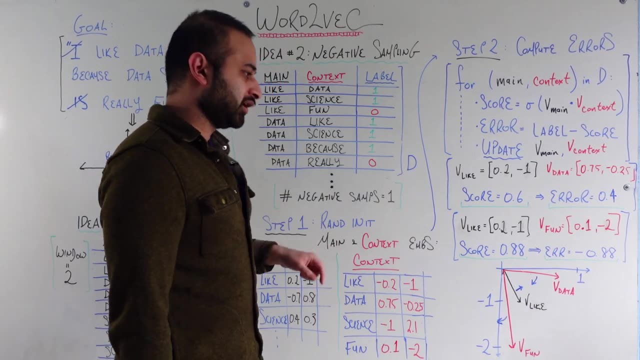 looking at each row one by one, And so the first row we'll look at is main word being like and context word being data with a label of one, and that's what we're going to do. That's what this example is going to talk about here. 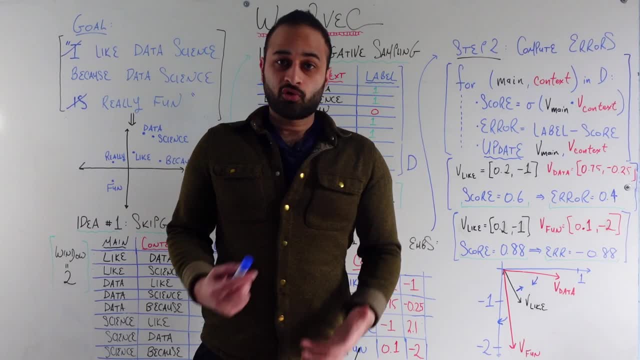 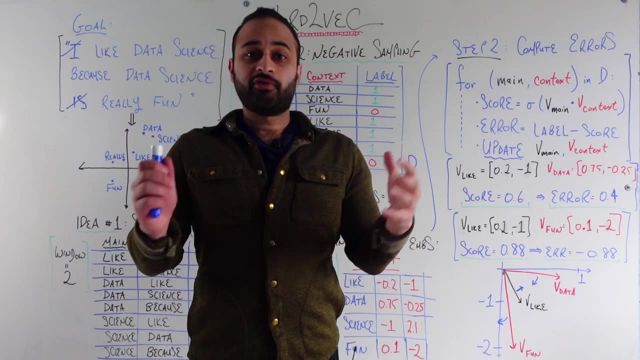 So the first thing we do is calculate something called a score. Now, the score is calculated as the dot product between the main vector and the context vector, and then you run the result of that through a sigmoid. Now, what does this actually mean? intuitively, 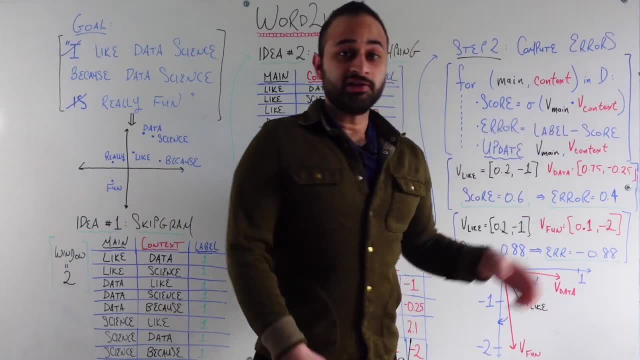 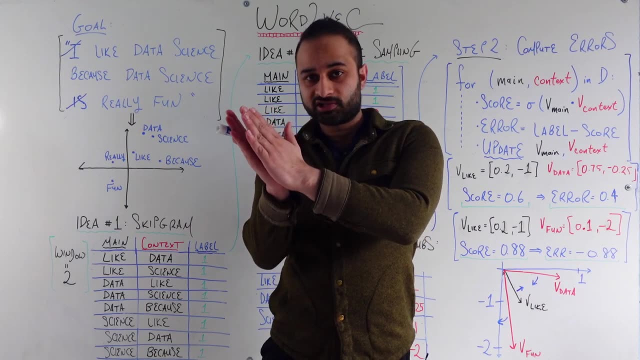 Well, let's walk through it together. If this dot product is very large, that means that the main vector we're currently looking at and the context vector we're currently looking at are close together in some sense in space, so that would cause the dot product to be large. 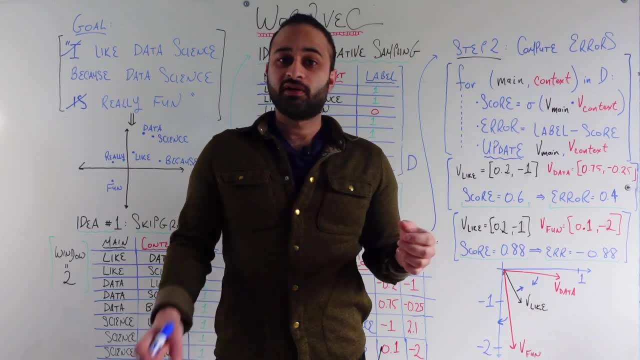 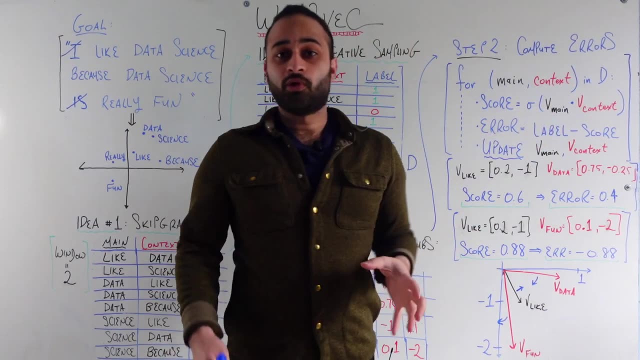 A large number put into a sigmoid function is going to give something very close to one. Remember, the sigmoid kind of squashes things between zero and one, and so if the argument in here is very big, we're going to have a score that's pretty close to one. 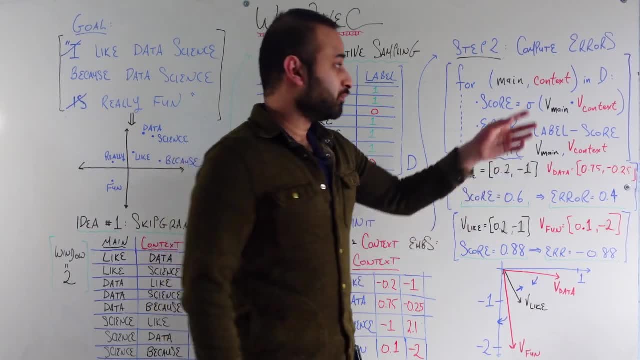 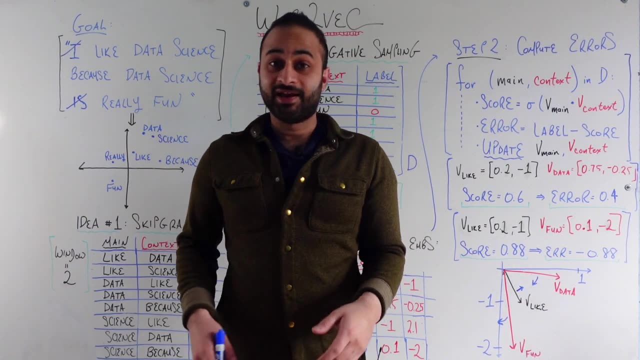 So a score being close to one is an indication that this main vector and context vector are close together in space. Conversely, if the dot product here is very negative, that means the two vectors are kind of opposite, facing in opposite directions, and so they're not similar. 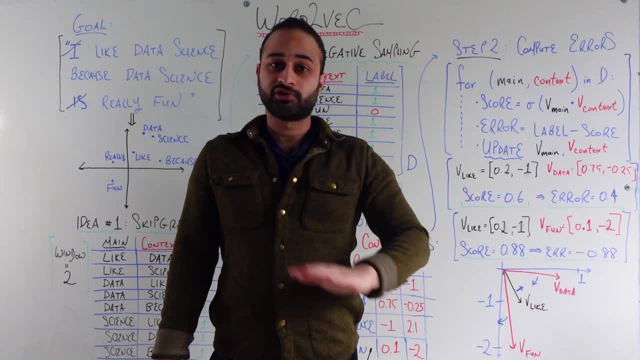 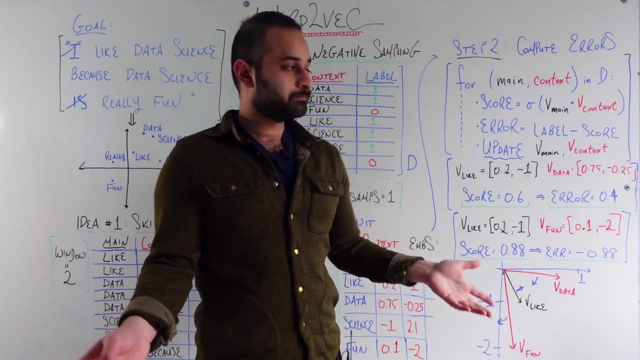 A very negative thing. fed into a sigmoid will give you something close to zero, and so the score, being close to zero, tells us these vectors are not very similar, not very close to each other in space, And so that's the first operation we do here. 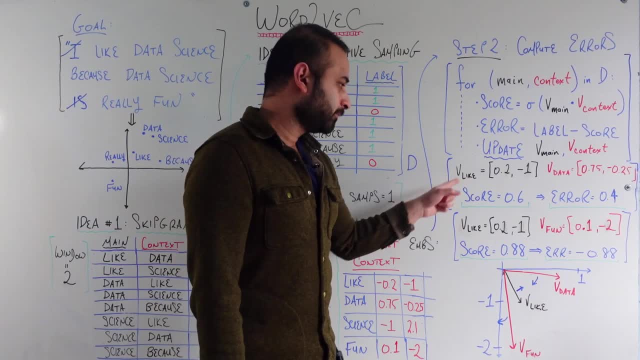 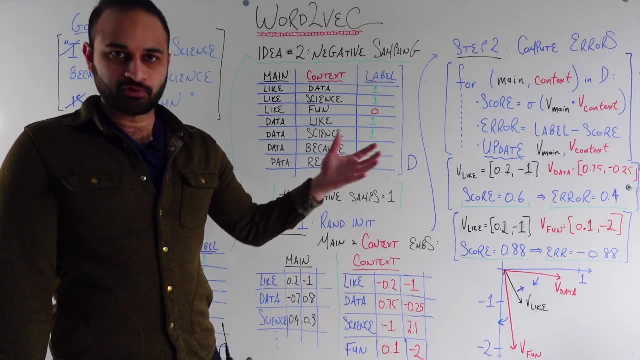 So we take the current embedding for the word like, which is point two and negative one. By the way, these are just randomly initialized values, so we're going to update these into things that make sense through this process. So the current main vector for the word like. 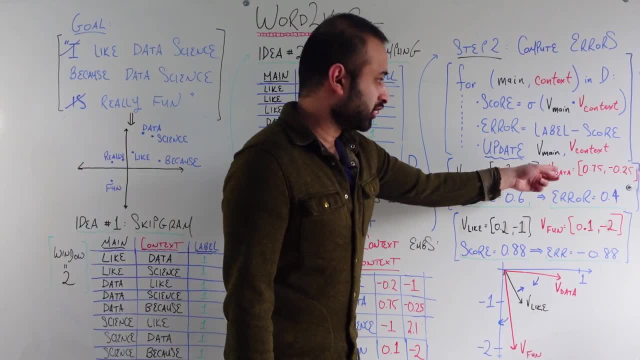 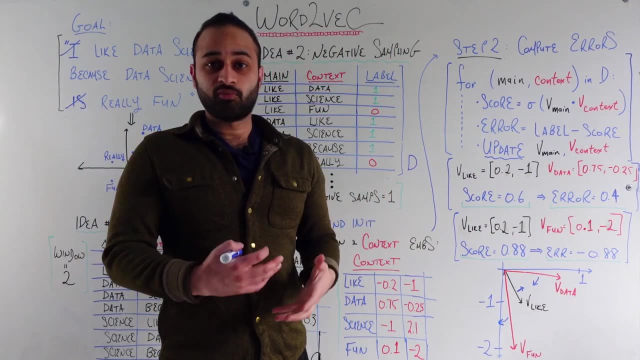 is point two and negative one. The current context vector for the word data, which is this guy, is point seven, five and negative point twenty five. We take their dot product, feed that into the sigmoid and so we get a score of zero. point six. 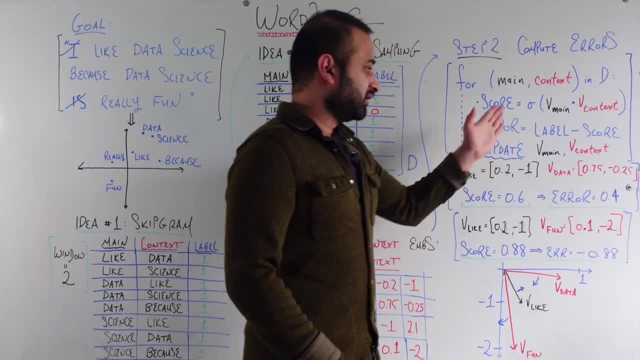 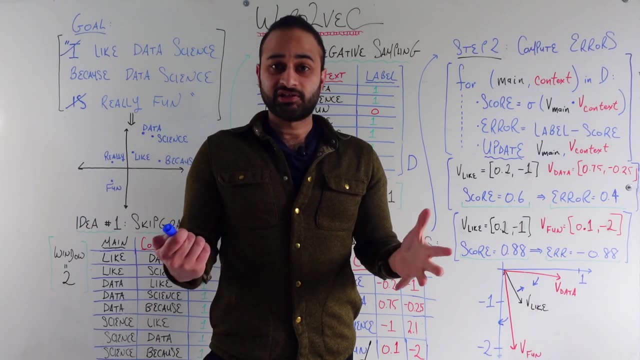 Now the next step is we calculate an error. The error is simply the label minus the score we just calculated. So the label here is one. Let's think about why this measure of error makes any sense If the label is actually one. remember that means that those two words 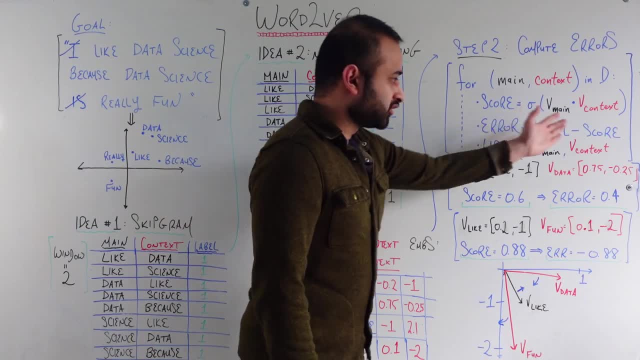 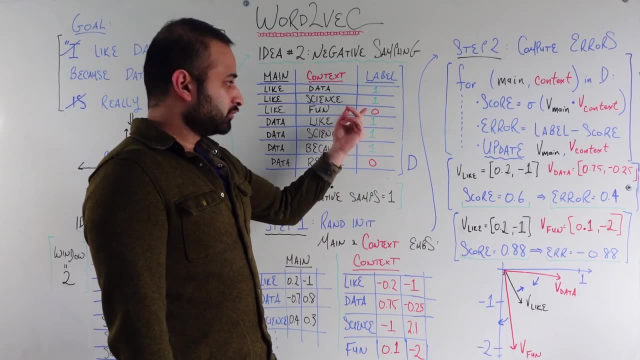 do actually appear close to each other, And so we would want the score to also be close to one, And that would cause the error to be zero. Now, if the label is actually zero, which means those two words do not appear in the same context, 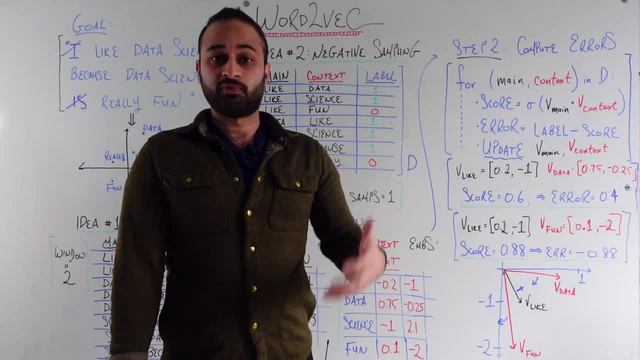 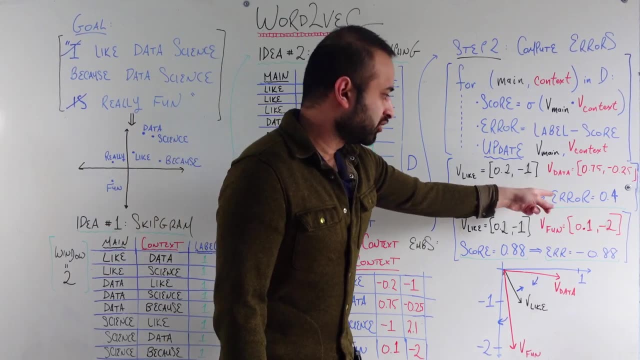 then we want the score to also be close to zero because, remember, a score close to zero tells the exact same story. So this measure of error does make sense, And if we do it on this example, we get zero point four, And so the fact that this error is positive. 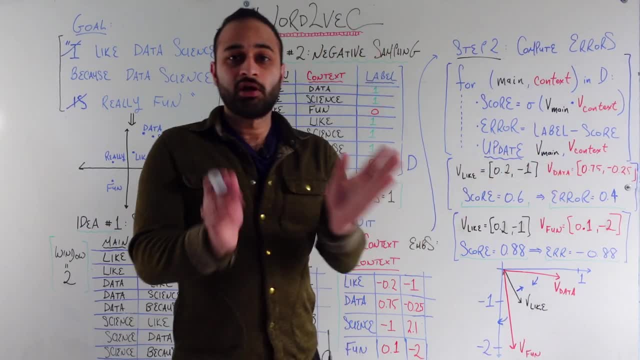 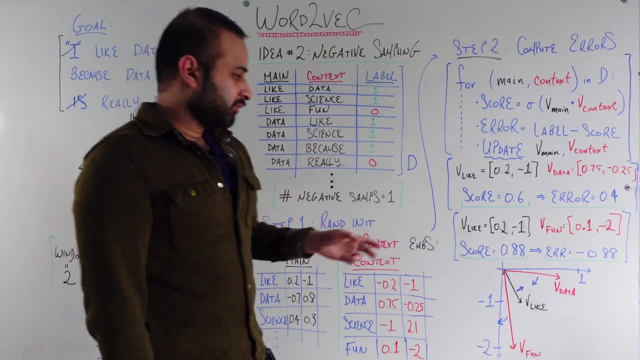 tells us that we want to move these two vectors closer together on the next iteration. Now, let's say we're looking at the third example here. Then we would have the main vector for like is again point two- and negative one, The context vector for the word fun. 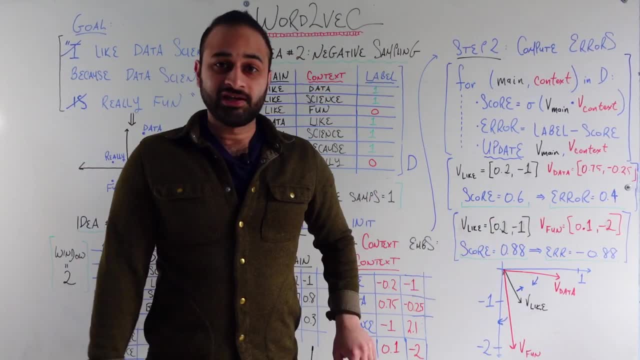 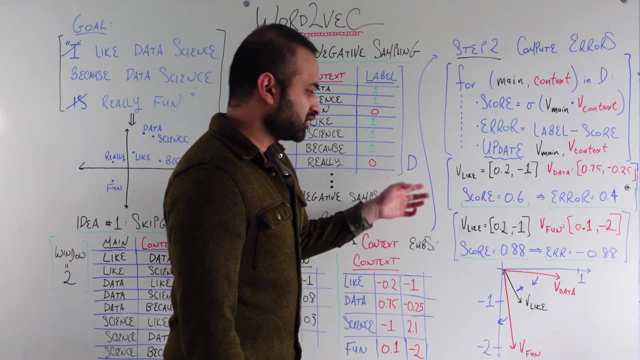 is point one and negative two. The score is zero point eighty-eight And the error is negative: zero point eighty-eight. The fact that the error is negative tells us that in the next iteration we would like to move these two vectors further apart, because they're not actually context vectors. 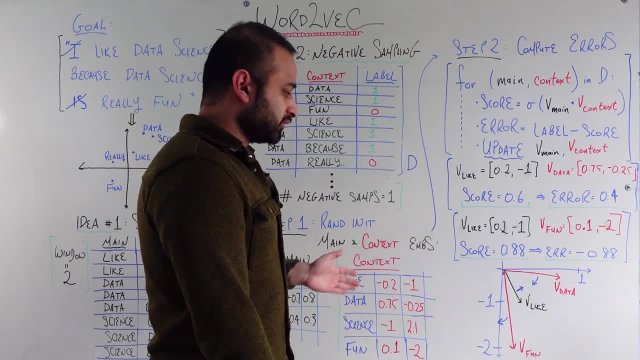 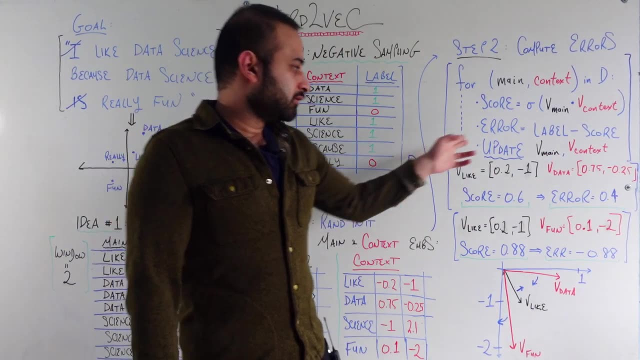 They're not close to each other in this sentence, And so that's exactly what we do in this diagram. So the last step we do here is we update the main vector and the context vector. And this word update, I've kind of left it intentionally vague. 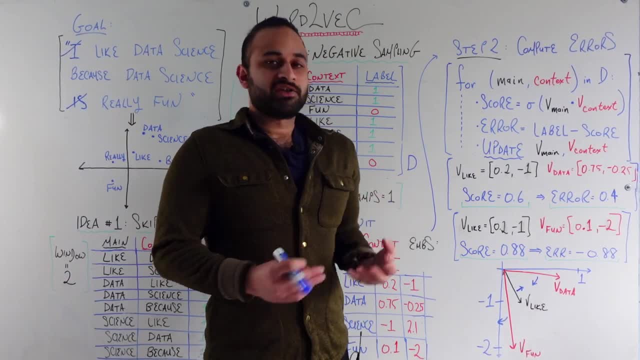 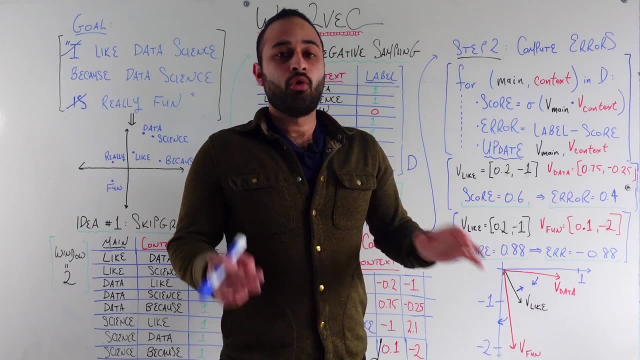 but there's a lot of different avenues you can go here. You can do something as complex as having a neural network behind the scenes and you're going to use these errors to update the weights and biases in the network. Or you can do something as simple. 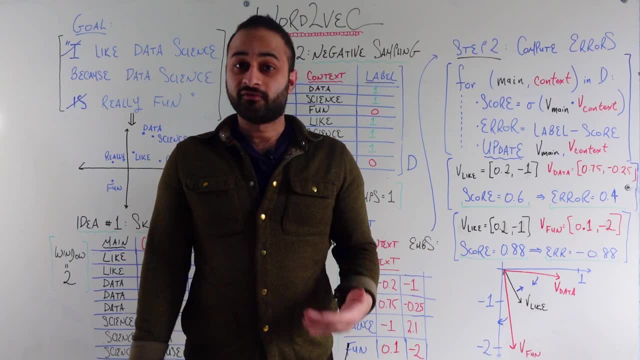 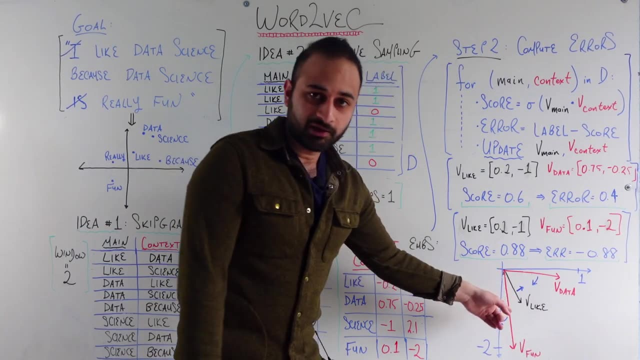 as literally just moving these vectors by a little bit in the vector space such that these errors are respected, And so that's exactly what's happening in this picture. So we have this main vector like, we have this context vector data and we have the context vector fun. 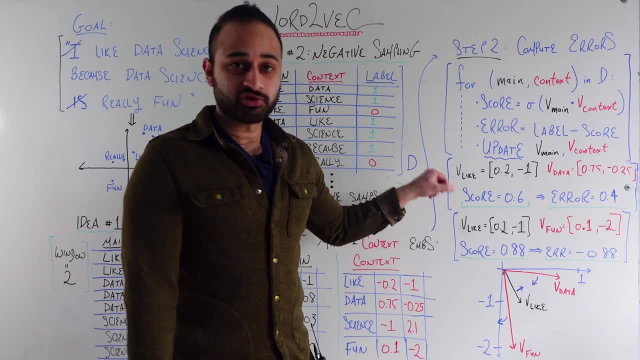 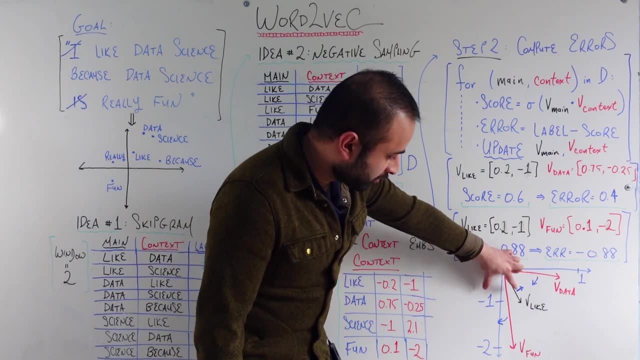 And, according to these errors, we need to move these two glies closer to each other. So like and data move closer to each other, And fun and like move further apart from each other, And so that is what will happen after one pass through all of these examples here. 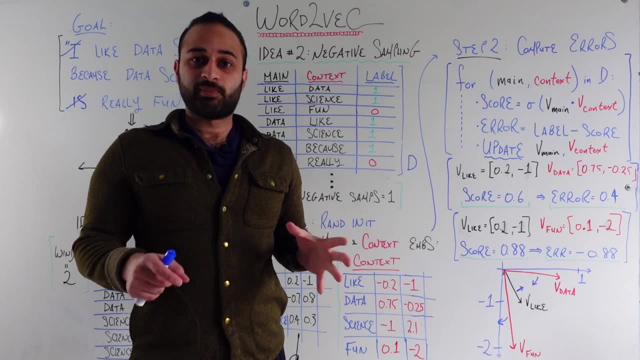 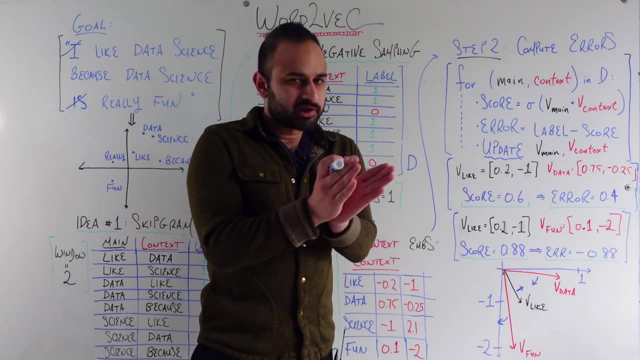 We're going to be delicately moving each of these vectors in the space, both the main vectors and the context vectors, such that things that are actually close to each other in their sentence end up a little bit closer to each other And things that are not actually close to each other. 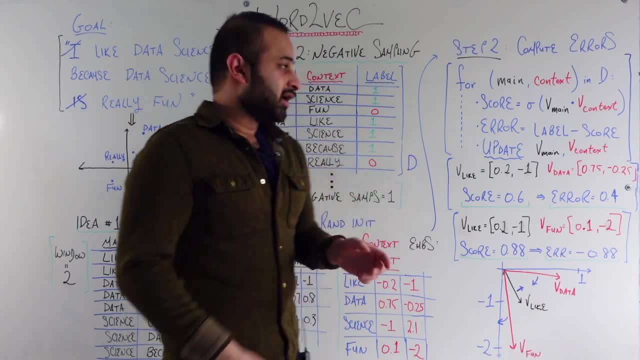 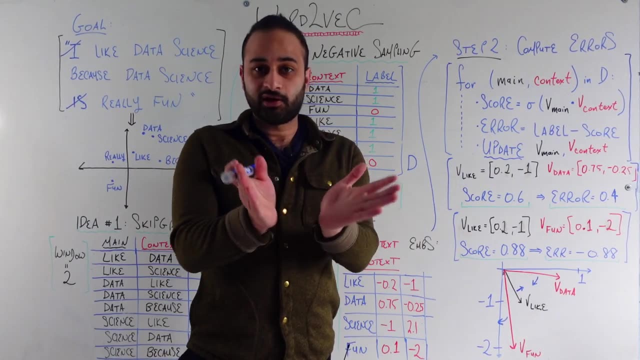 in the sentence end up a little bit further from each other, And then we can just repeat. We can go through this data set as many times as we would like And each pass through there. we're just going to be doing these steps again and again, and again. 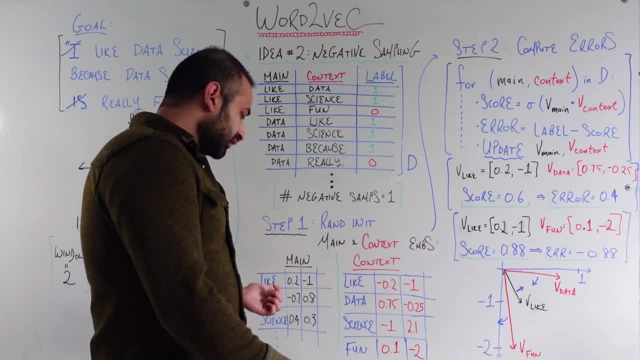 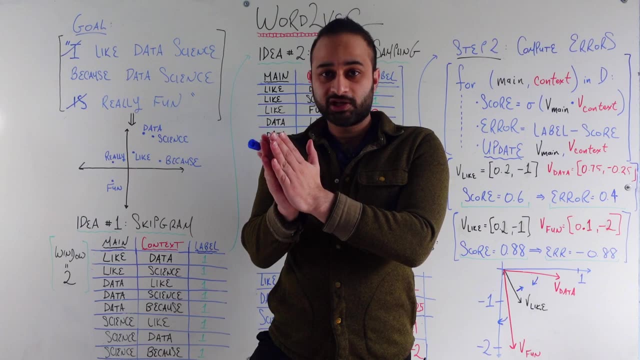 So that, at the end of the day, these main embeddings end up in such a position that words that are close to each other end up literally close to each other in the vector space, And words that are not close to each other in the sentence end up literally far from each other in the vector space. 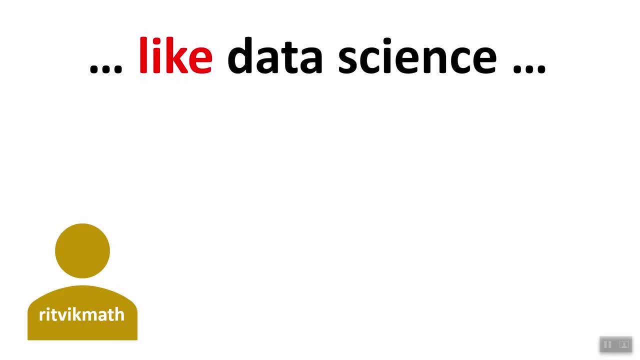 So it's a very, very interesting technique. I think- Hey, sorry, Ritvik from the past, This is Ritvik from the future. when I'm editing this video, I just wanted to make sure I get the point across about why this works really fast.